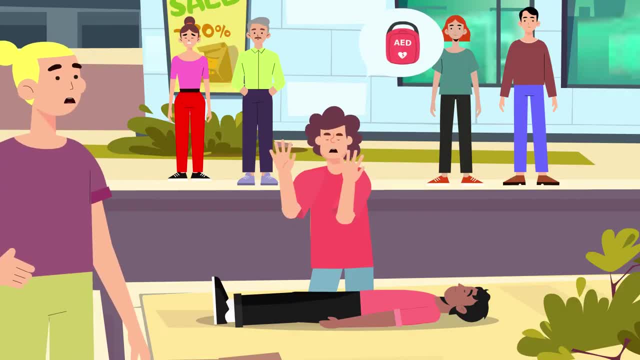 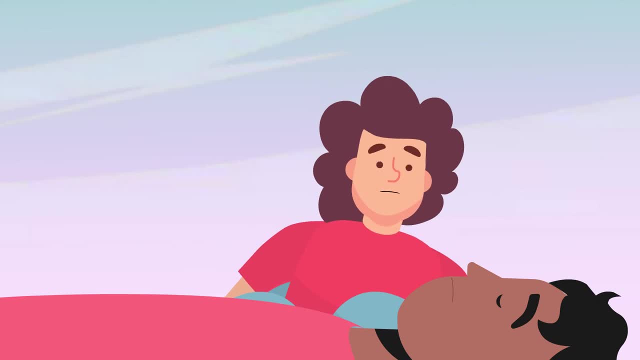 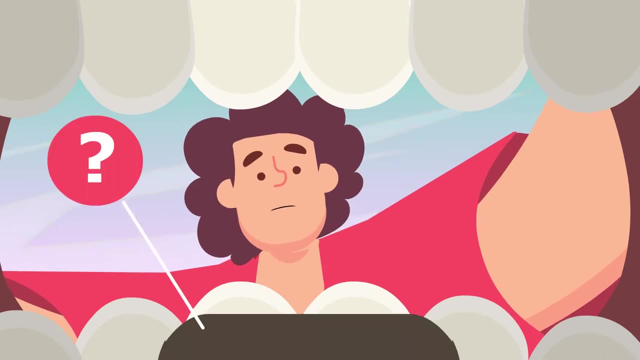 bystanders for help and send for defibrillator, if one is available, while waiting for the paramedics to arrive. move on to the airway. is the person's airway clear? you need to check their airway by opening their mouth and having a look inside. if you find any obstruction whilst checking the airway, 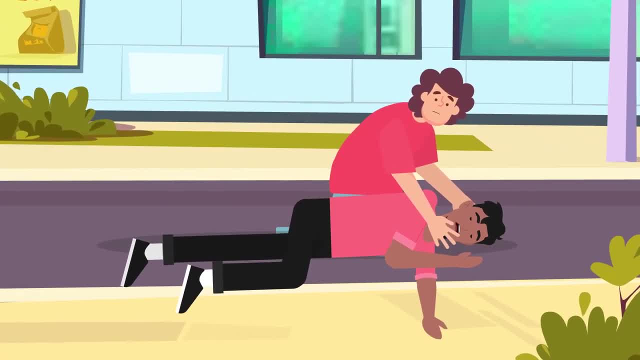 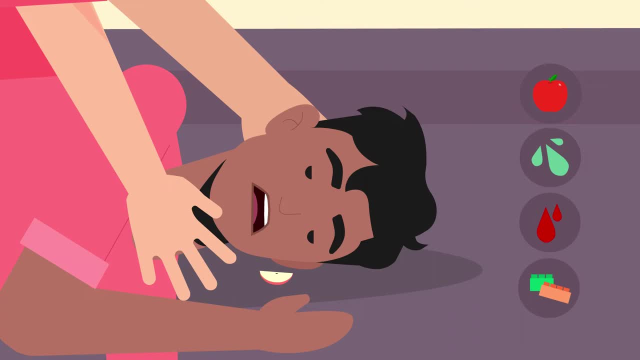 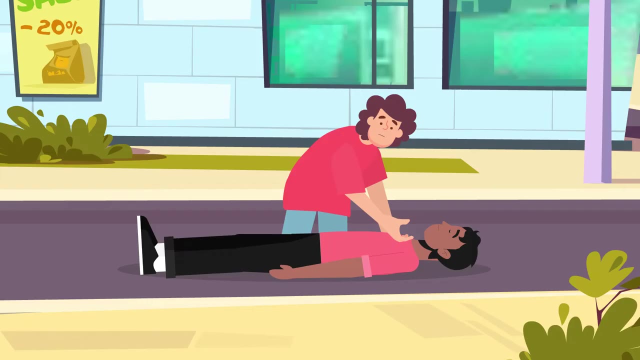 roll the person onto their side to clear the airway of any foreign material, such as food, vomit, blood, toys, by letting it drain or gently sweeping out the foreign objects. once the obstruction is clear, reassess for responsiveness and normal breathing. if their mouth is clear, tilt their head gently back and check for. 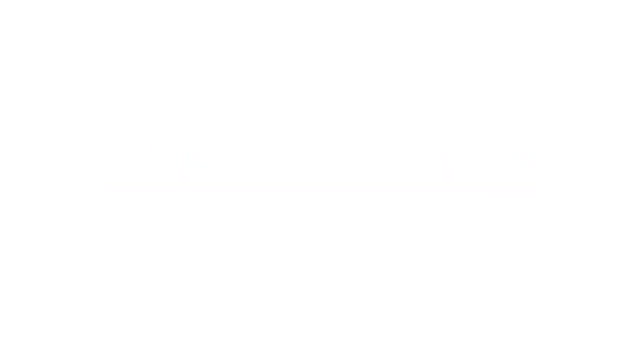 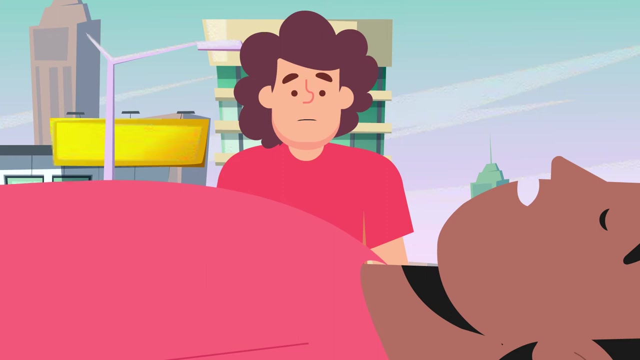 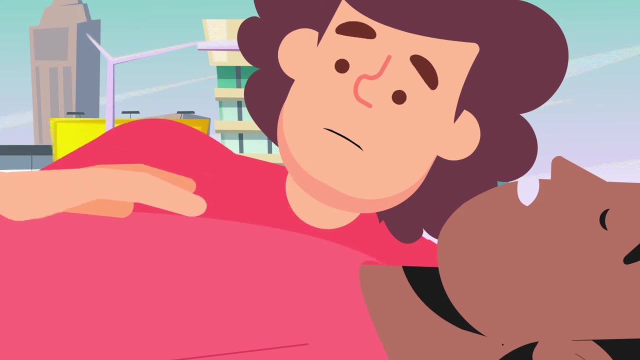 breathing. breathing. check for breathing using the look, listen and feel method for 10 seconds: look for the rise and fall of the chest. listen for normal breathing by putting your ear near to their mouth and nose. feel for breathing by putting your hand on the lower part of their chest. 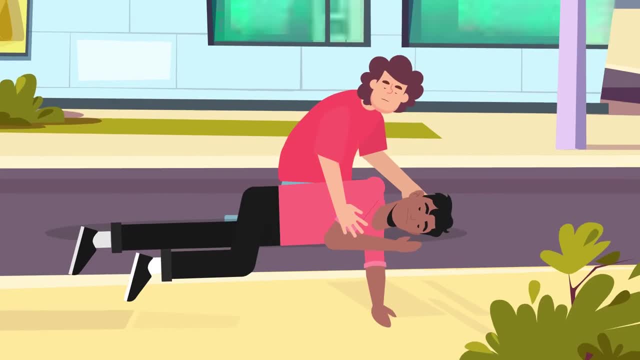 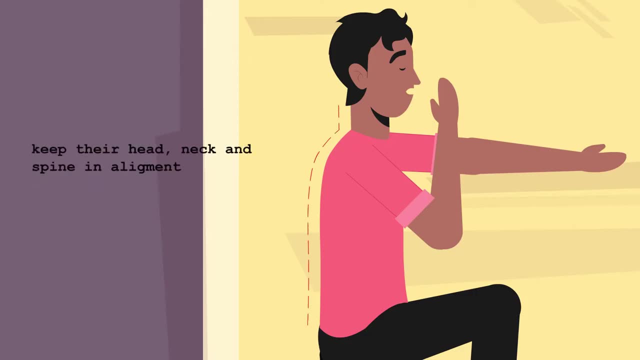 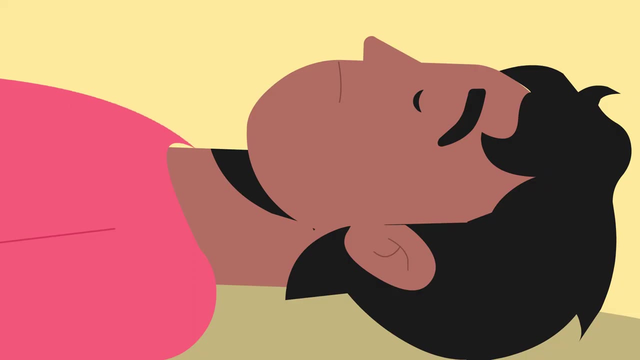 looking and feeling for the rise and fall. if the person is unconscious but breathing, turn them onto their side carefully, ensuring that you keep their head, neck and spine in alignment, monitor their breathing and manage any injuries until the paramedics arrive. if the person is not breathing normally, start. 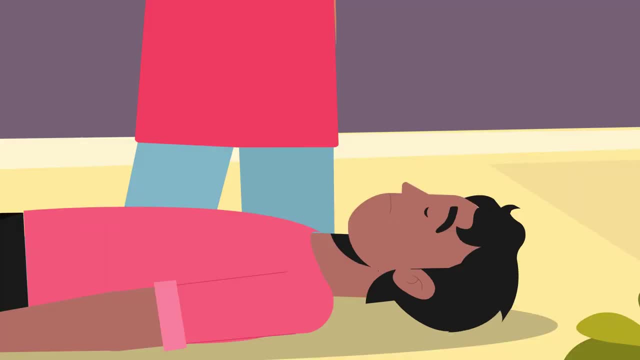 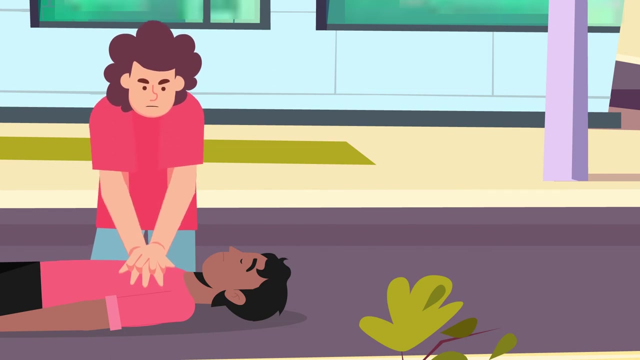 CPR immediately. make sure the person is on a hard surface. face up on their back then place the heel of one hand in the center of their chest, your other hand on top. press down firmly and smoothly 30 times, roughly two compressions per second, or about 100 to 120 compressions per minute, followed by giving two rescue breaths to get the 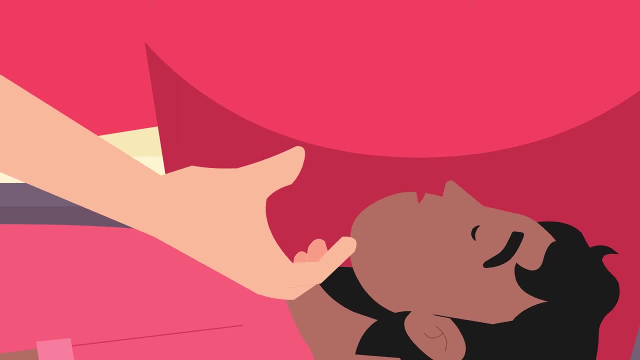 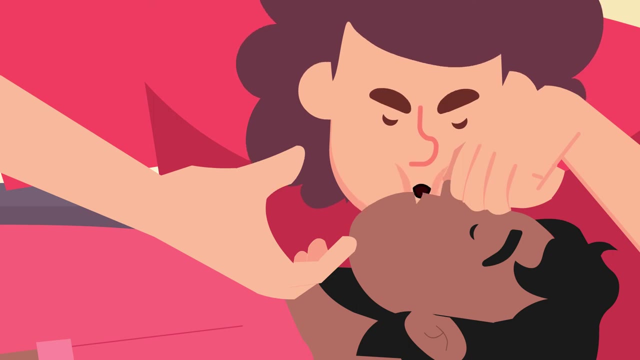 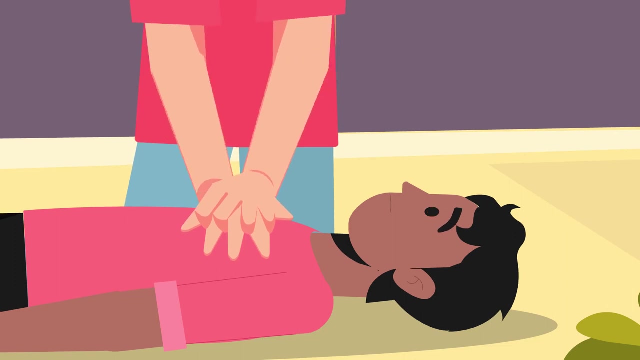 breath in. tilt their head back gently by lifting their chin. pinch their nostrils closed. place your open mouth firmly over their open mouth and blow firmly into their mouth. continue this sequence until the person responds or the paramedics arrive to take over, if the person is still. 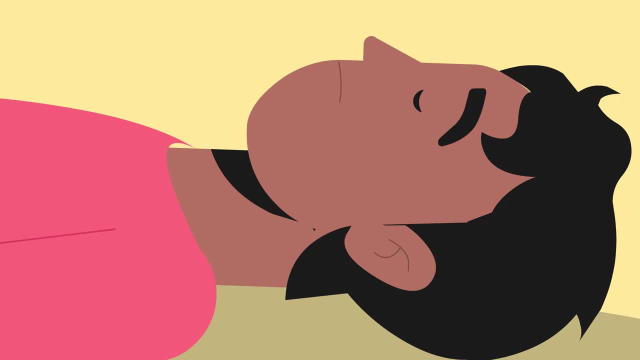 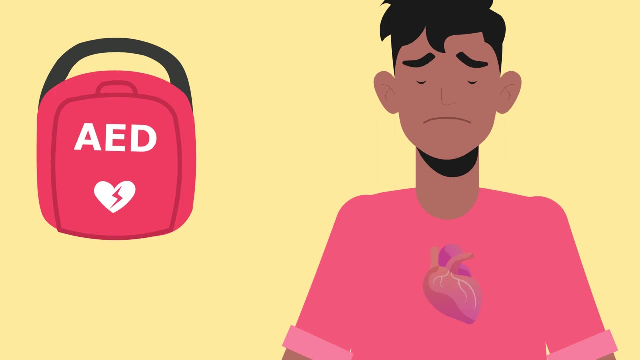 unconscious and not breathing. the defibrillator should be applied as soon as it arrives. d for defibrillator, defibrillator, or aed for short meaning, automatic external defibrillator, is an easy-to-use medical device that analyses the heart rhythm and, if required, deliver an.